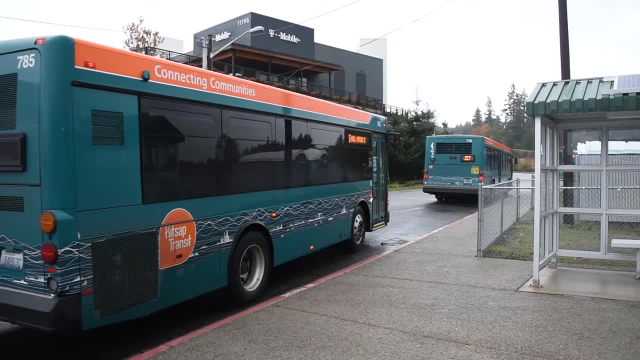 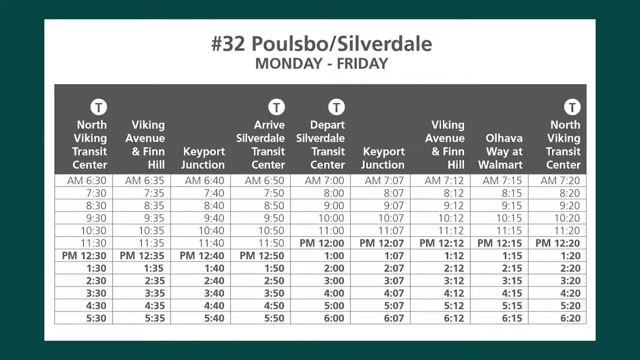 we'll call this a simple schedule. A second type of schedule we have is a long layover. For example, Route 32 includes a 10 minute layover at the Silverdale Transit Center to allow customers to make other bus connections. A third type is a ferry connector. that includes ferry departure times in the far right columns. 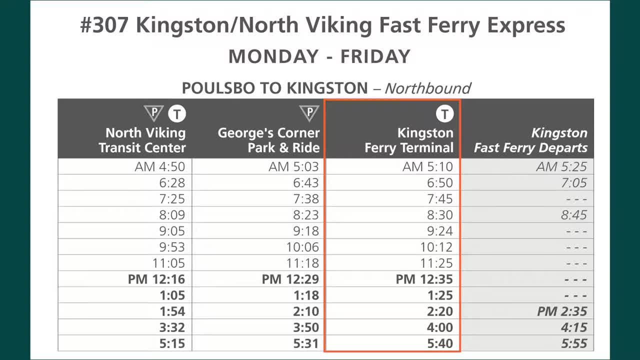 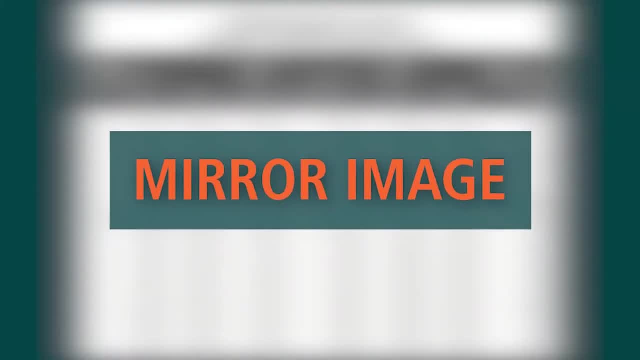 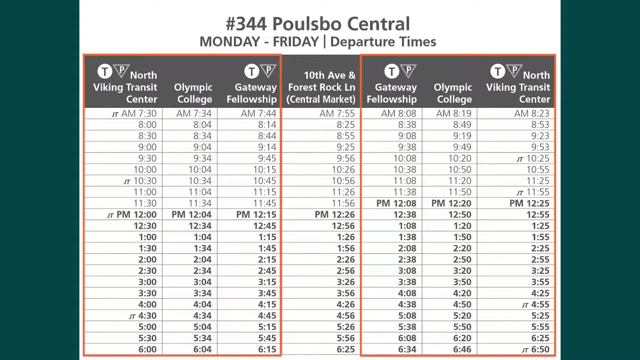 and the arrival times for the bus stop that connects to the ferry in the second to last column. Then there is the mirror image type, like Route 344, which has a stop in the middle and then stops at the same time points going back. the way it came. Reading left to right is important here. 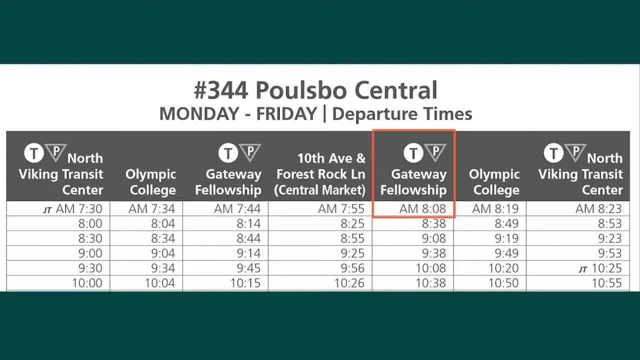 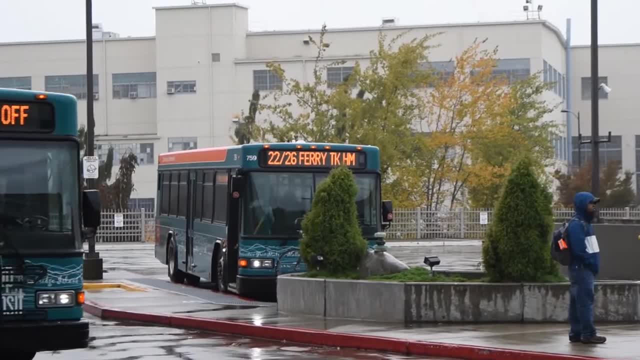 For example, if you need to get to Gateway Fellowship at 8.08 am, you should wait at your stop at 7.55 am to catch the bus traveling from Central Market to Gateway. And the last type we'll call dynamic schedules, which operate differently depending on the time. 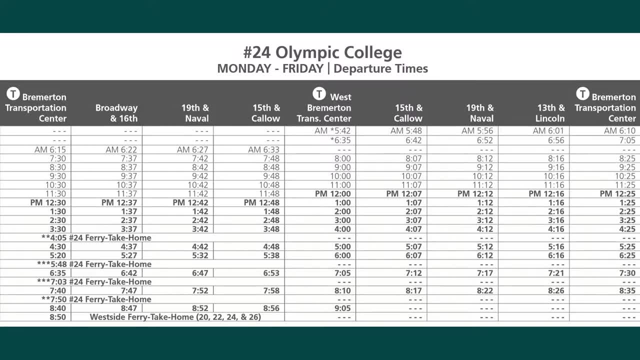 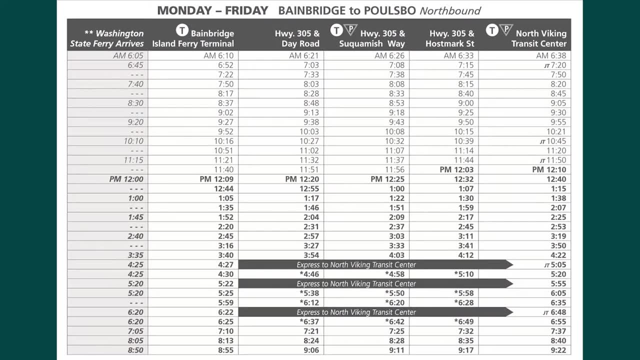 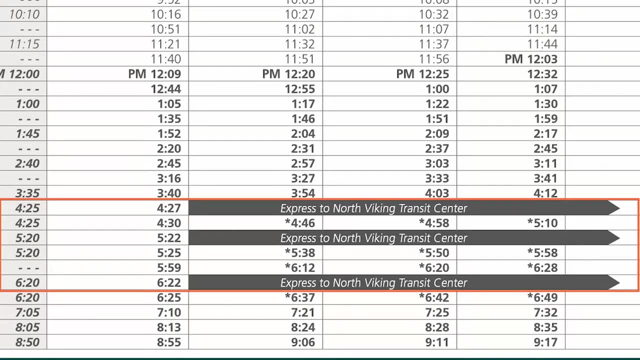 of day. During the afternoon commute hours, Route 24 operates ferry take-homes that only drop off passengers at the stops they request. Also, during commute hours, Route 390 operates express routes in the early evening that take passengers to North Viking Transit Center without making any stops. 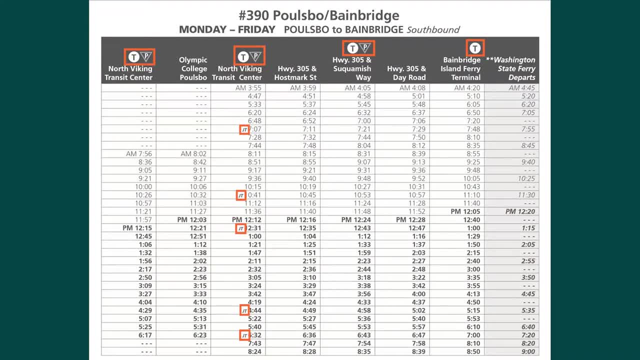 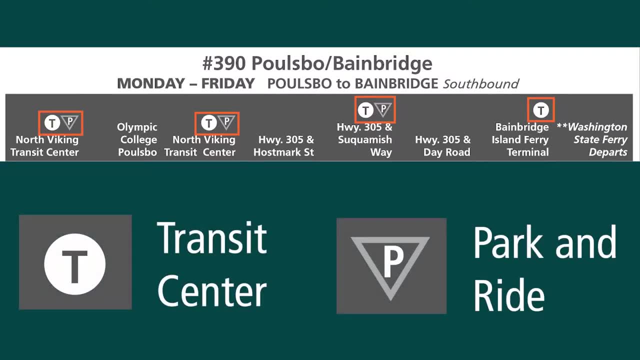 You will sometimes see symbols in the timetables that indicate unique features at some of each route's busiest stops. The T symbol indicates that the stop is a transit center or a transfer point, while the P indicates that the stop includes a park and ride you can leave your car at to. 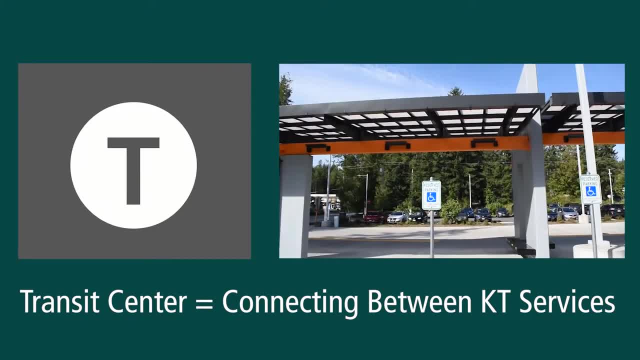 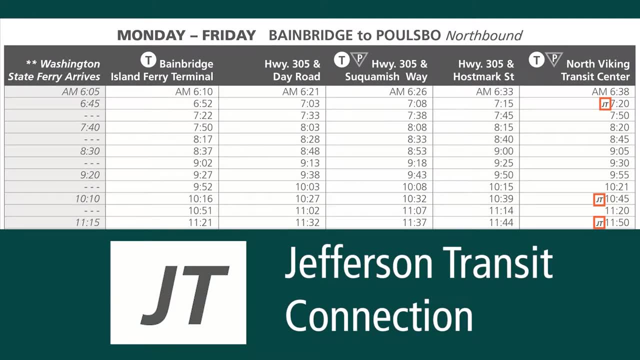 take the bus. A transit center is a bus stop you can use to transfer to a different bus or to a ferry, if applicable. The JT symbol next to these time points here indicates that you can connect with a Jefferson Transit bus at these specific times. Going over to the. 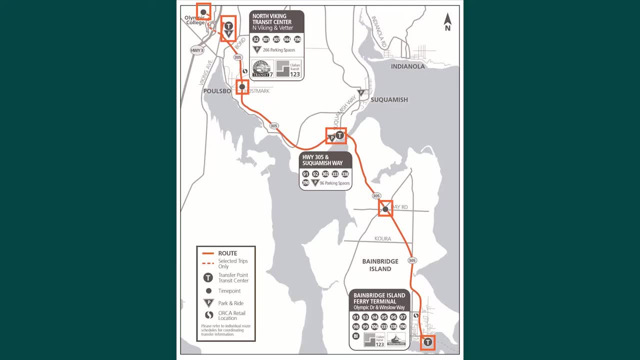 map. you will see six dots that represent the stops in the timetable, which in this case includes the route's two transit centers and a smaller version of a transit center called a transfer point in the middle. Note that there are many stops not shown in between the ones shown on. 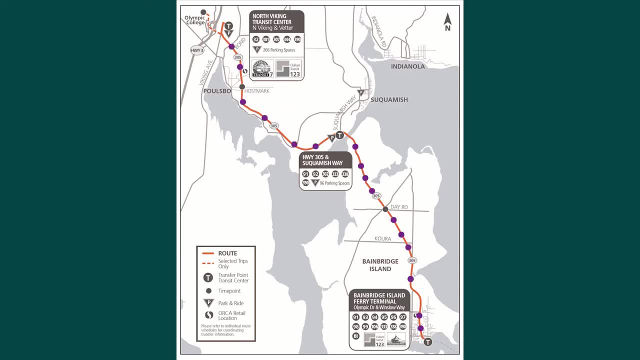 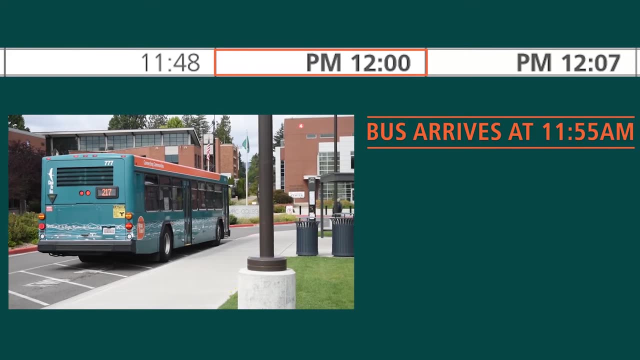 the map. but what makes time-pointed stops unique is that bus drivers must wait at these stops if they arrive early. For example, if a driver shows up to the stop in the middle at 11: 55 am, the bus has to wait for five minutes before departing at the scheduled time of 12 pm.